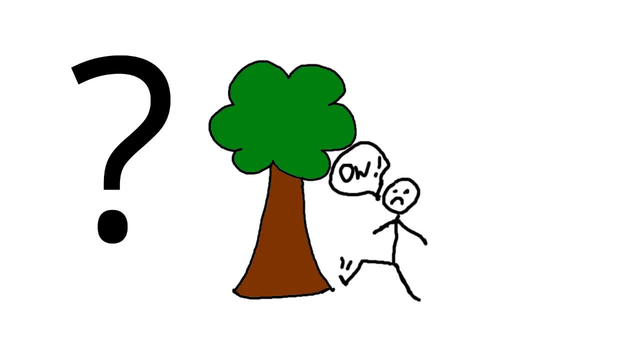 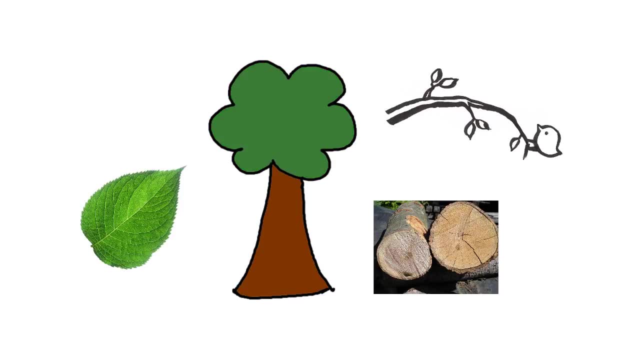 foot. now why is that? it's just because the materials are different between the two, and the shapes of them are different, and how they respond are then different. so the trunk of the tree is made out of hardwood, while the leaf is made out of much softer plant material, right? 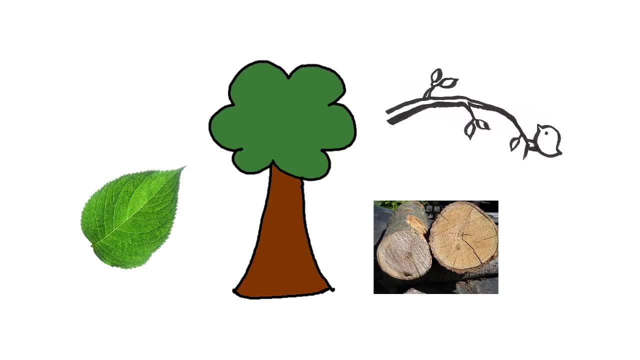 so breaking this tree down into even more basic components. you've got the geometry of the tree, so you have the general shape, and then you have these materials. like i mentioned before, and within the fe modeling world, these two things are really important, so the geometry can be files that just 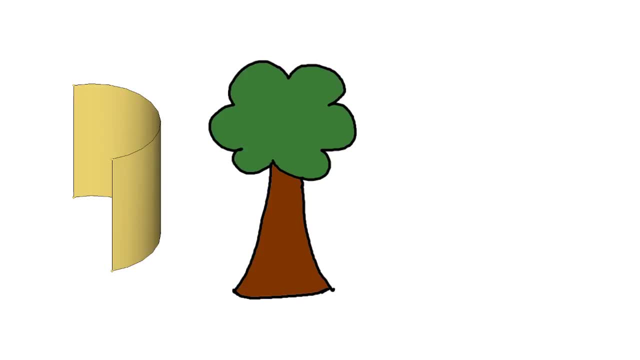 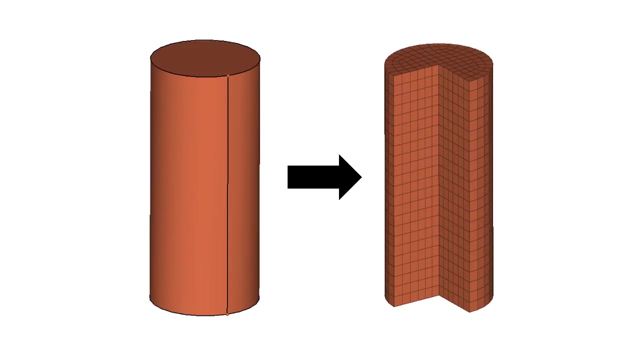 represent the geometry like stl files or cad files- if you've heard of cad- and the materials are then represented in something that's a little higher than this topic right now. but let's just consider that you have a filler that fills the geometry and you can 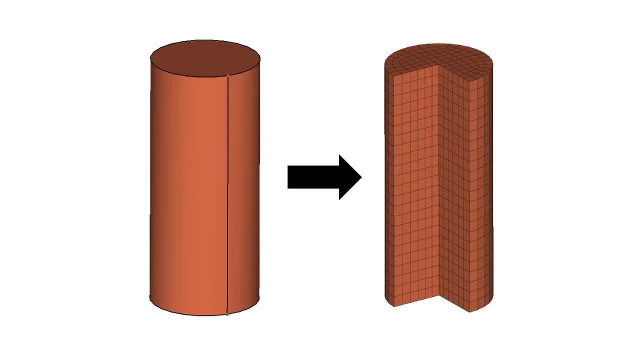 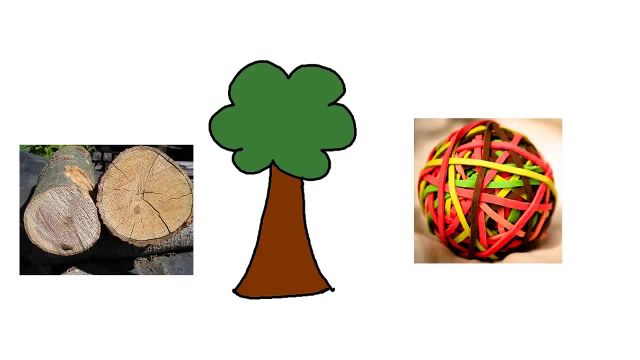 give that filler different material properties, so you can give it the properties of steel or the properties of rubber. so in the fe world you can give this tree the properties of wood, like an actual tree, or you can give it properties of rubber. and if you actually give the tree properties, 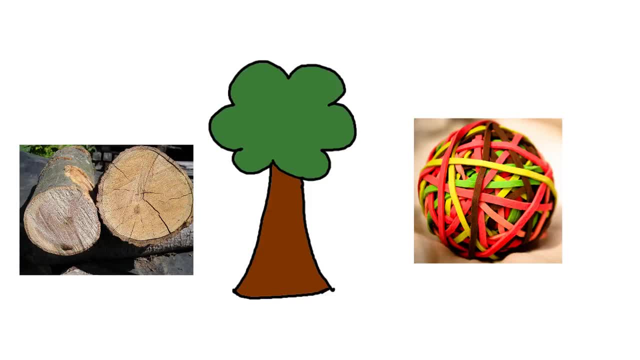 of rubber, then it's going to bend like rubber, so that's. a benefit in the fe world is that you can just manipulate things however you kind of want to and see what happens. this filler is what we call a mesh, so if you hear the word mesh, we're 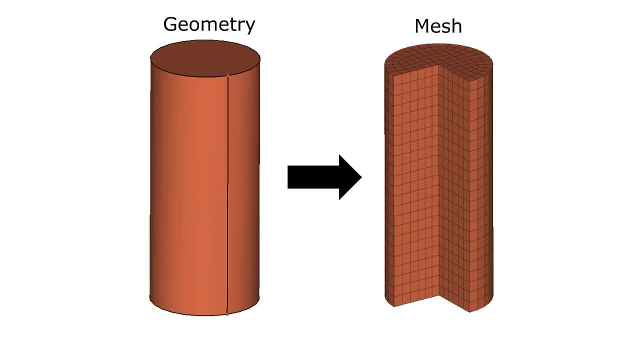 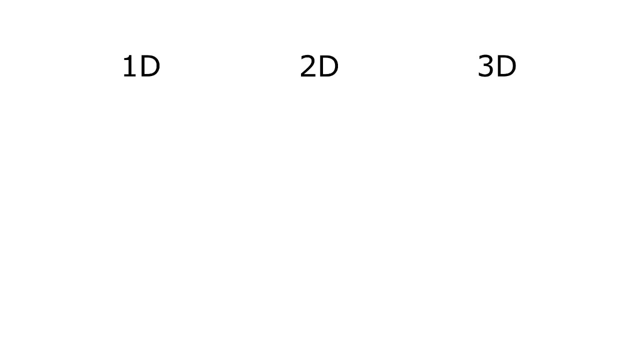 talking about this finite element tool that fills the geometry of an object, and this mesh is made up of different types of what we call elements. these elements can be one-dimensional or two-dimensional or three-dimensional, and within each of these dimensional elements, there's a lot of different types of elements that can be used to fill the geometry. 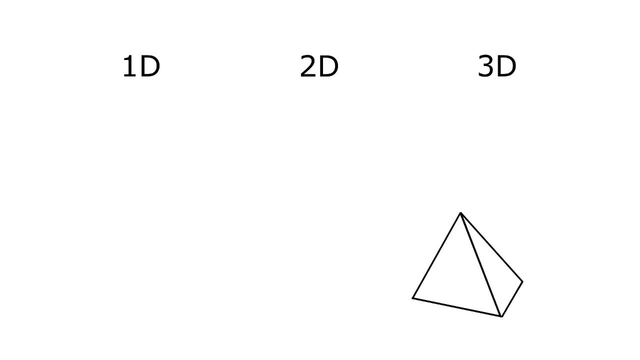 you have different types. so you can have pyramidal elements, you can have block elements or just squares or beam elements, all these different types of things that can be used in their own specific applications. so you can use beams to represent like a pole, you can use shells. 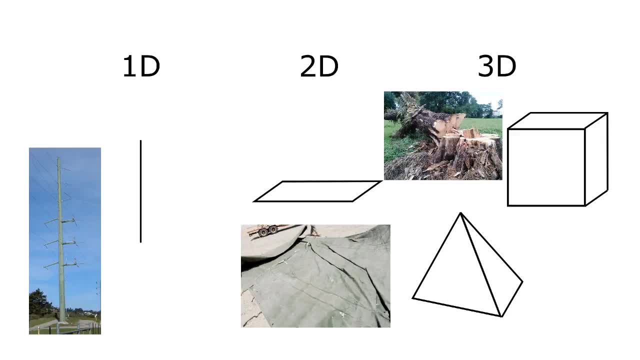 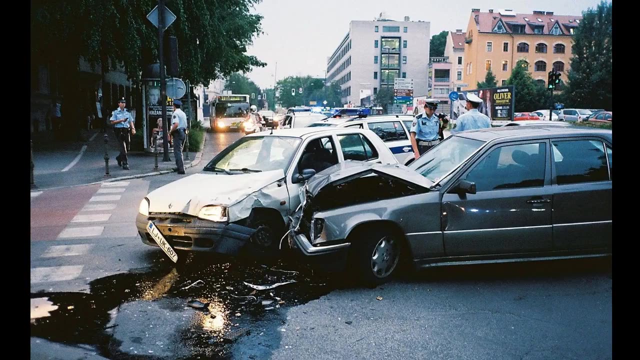 to represent, like a coating over something, and you can use solids to represent something that's going to deform through the object, like this tree. so, moving away from this tree application, we can relate this to a more real life application. so let's think of a car crash. okay, companies have to pay lots of money to do yearly. 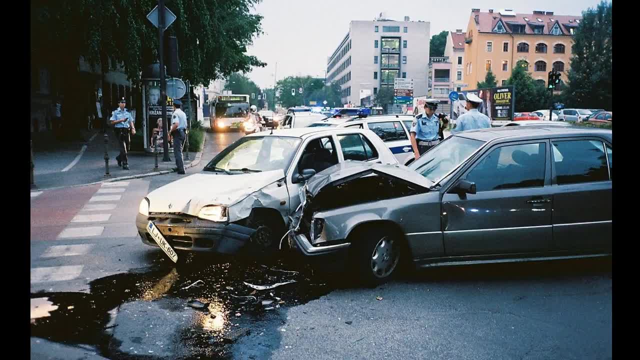 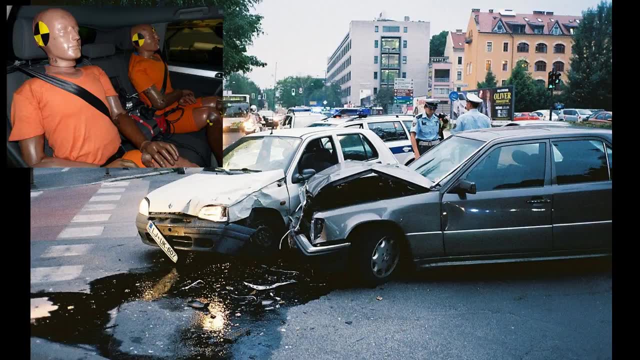 car crash evaluations and evaluate how safe their vehicles are. and to do this you have to instrument these cars. these dummies and the dummies themselves are expensive and it takes all day to instrument them. then you crash this car that's worth thousands of dollars, and they do this to make sure that the 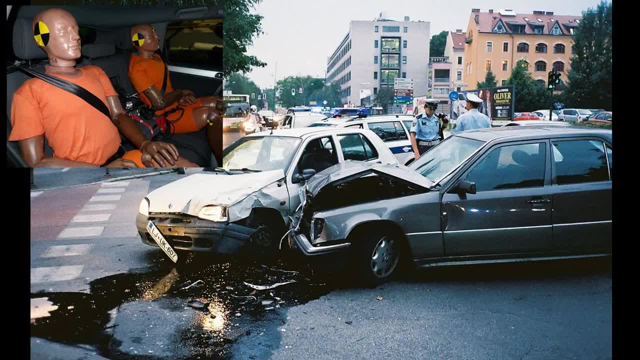 cars are safe and within this there's just a lot of different types of elements that can be used to create a car crash. it's a lot of money. what you can use fe for is you can make a model of a car, which pretty much every automotive manufacturer in America has done, and they take these car models. 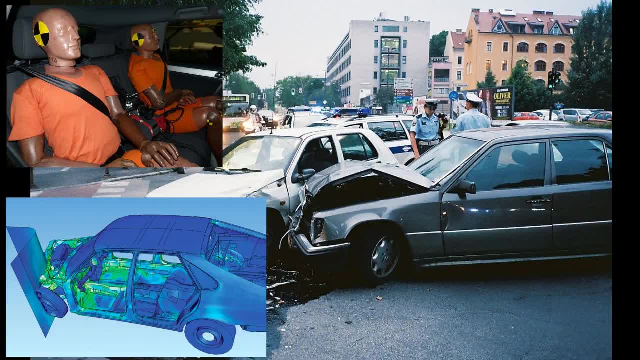 and then wreck them through fe, and what you can do is, instead of wrecking a physical car, you can wreck the model of a car and see how the car responds. so the first part of finite element analysis is developing a representative model of what a real life object is in the media, actual location. so 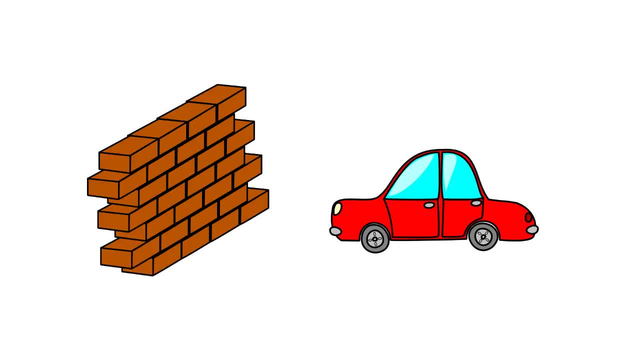 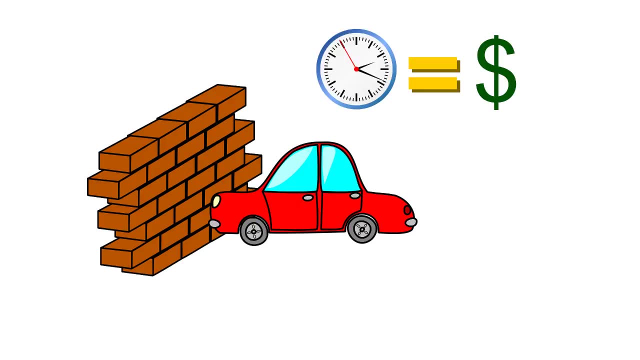 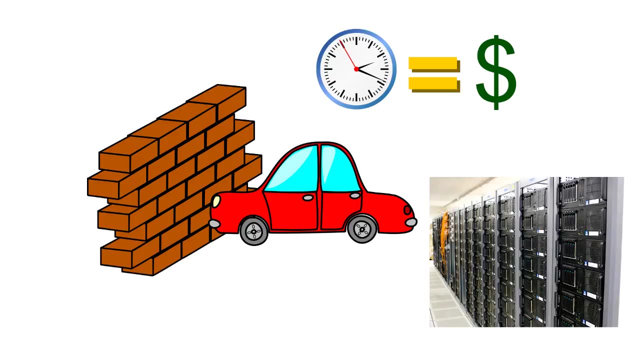 going to do when it is met with a specific boundary condition. So the benefits of this are that once you have the model, it's much cheaper to use than doing physical tests. It's much faster. However, you do sometimes need higher amounts of processing power, so you need some pretty 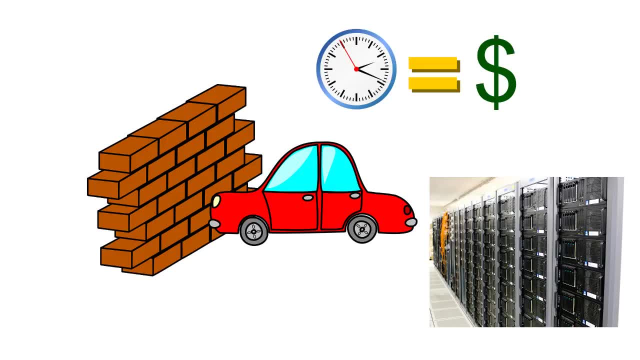 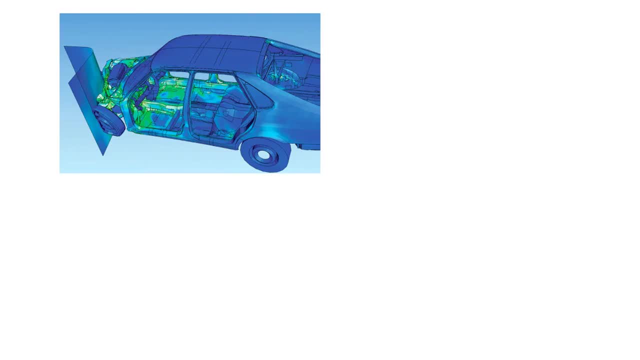 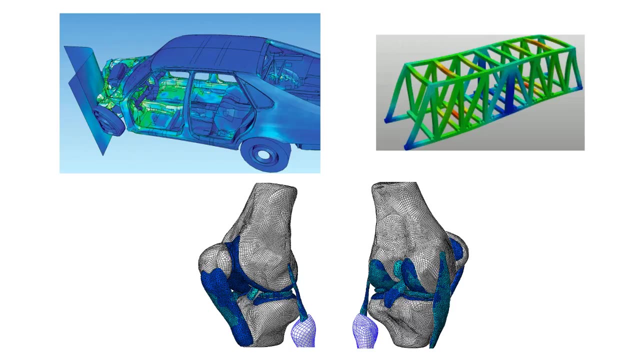 powerful computers And applications in the field of finite element analysis include, like I mentioned, automotive manufacturers, automotive crash tests, civil engineering like bridge tests, weight-bearing tests and even in the world of human body models, which is actually what I work with. 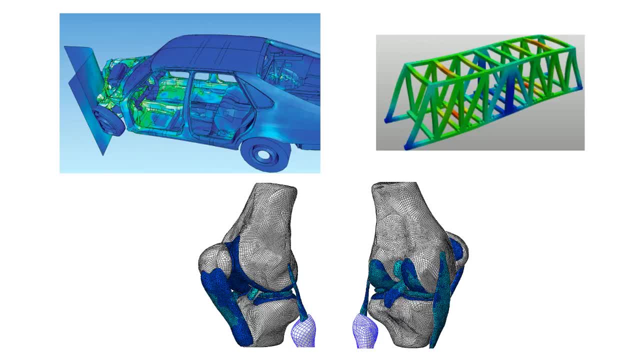 And it's really complex And it's pretty much limitless in the field of finite element analysis is growing and it's a good field to get into. However, there is a large learning curve and this is just a really basic level intro to this.